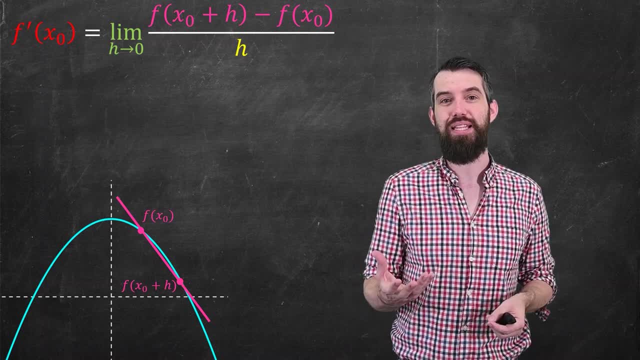 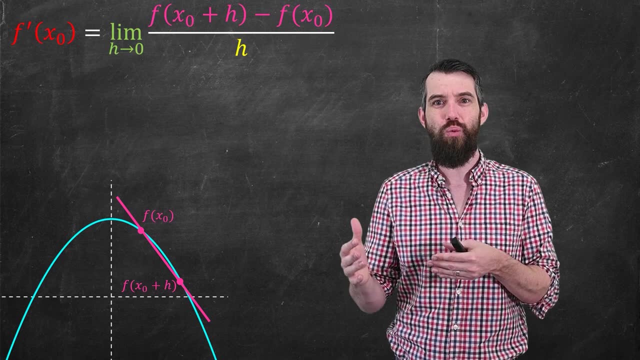 the point x naught, f of x naught, and x naught plus h, f of x naught plus h. You have those two points that go between them, And then what's the value of the h? Well, the h represents this width. on the. 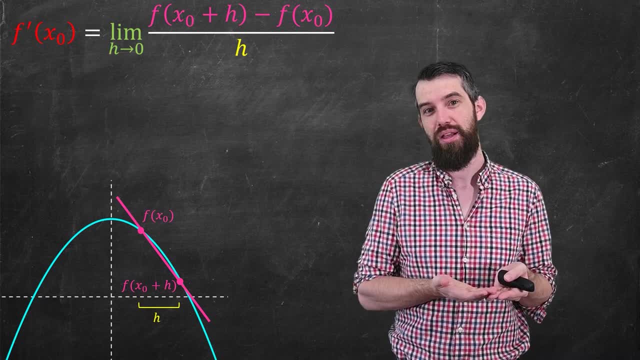 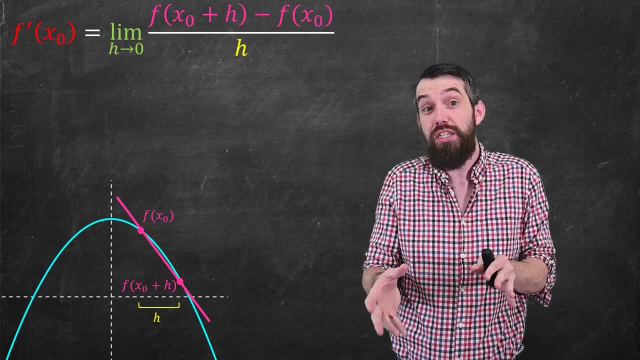 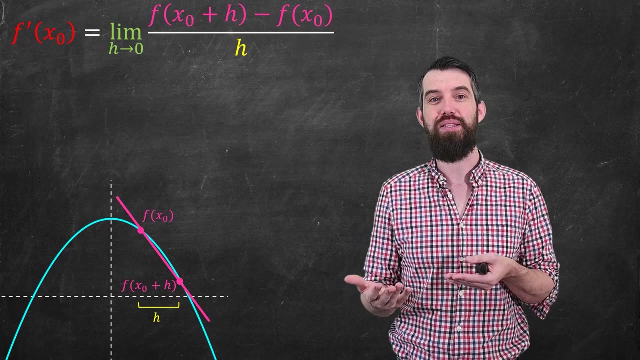 x-axis. that represents the, the change in the run, if you will. So the slope of that secant line is rise over run. That is what the difference quotient represents. It represents the slope of the secant line. And then the limit says: well, what happens if the x naught plus h and the x naught? 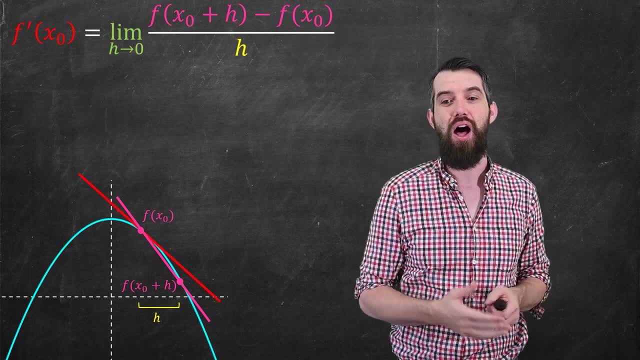 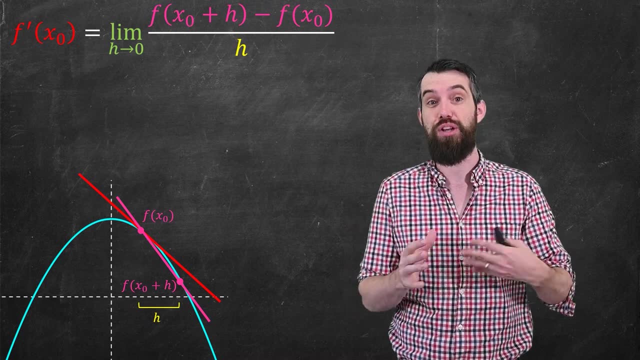 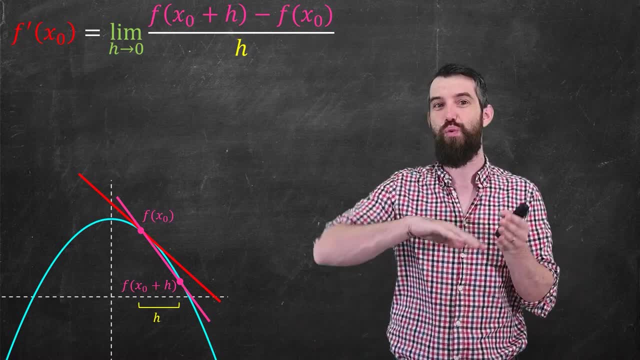 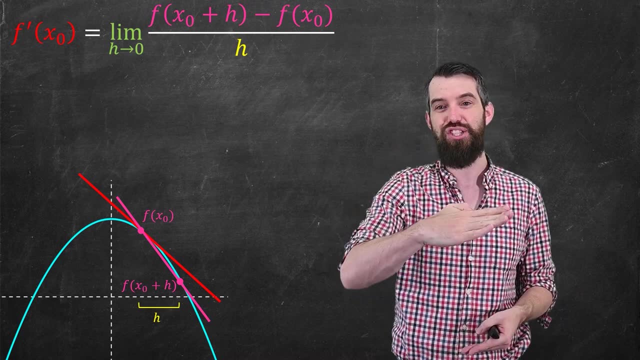 to be differentiable And it meant it was relatively nice. You didn't have any sort of weird sort of cusps or jumps or spikes or anything bizarre happening at this point. x naught because you could sort of put this nice tangent line on and just come along and kiss the curve. The curve had. 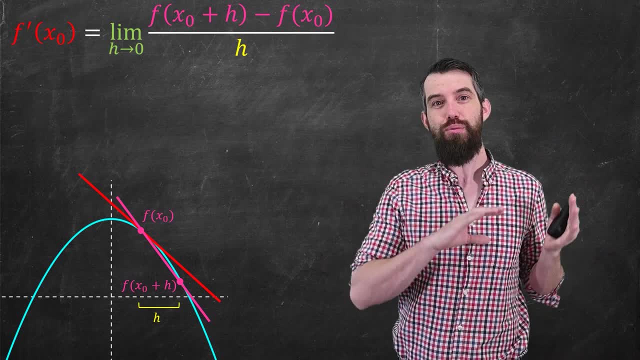 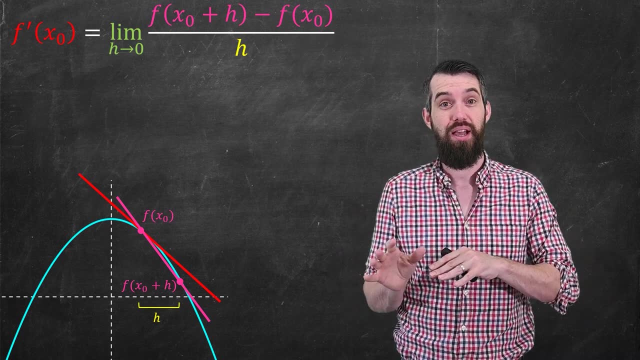 to be relatively nice for this to be able to occur. So that was one view of differentiability, Probably the most common way that it was presented. But I want to take a different view of differentiability of a single variable function. I'm going to take this limit expression and I'm going to just sort 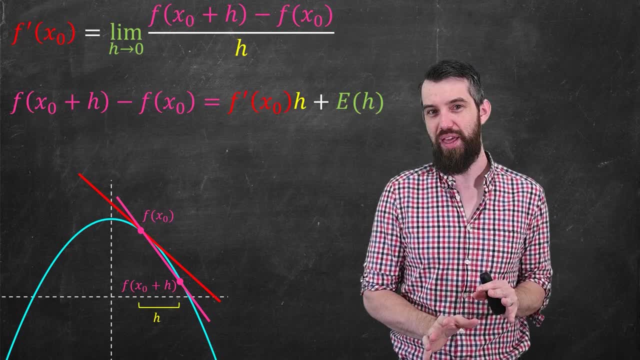 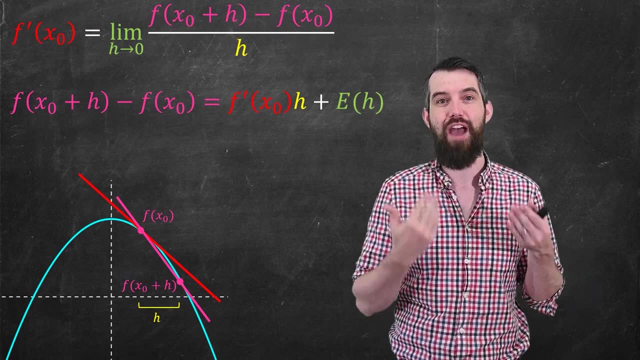 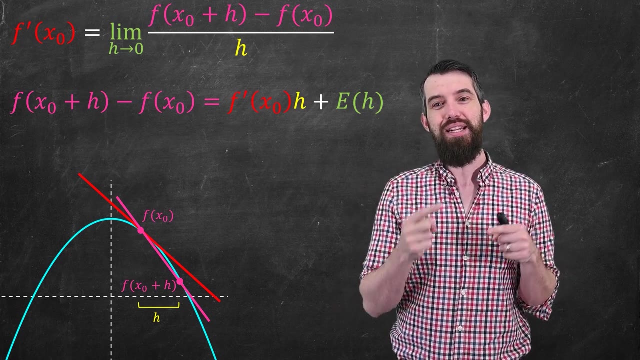 of rearrange it a little bit. It really looks almost the exact same thing, but a few little details have changed. So first thing I did was I took the h on the bottom and I multiplied it up, so I had an f prime of x naught times an h, And then, in place of a limit, what I did instead was write: 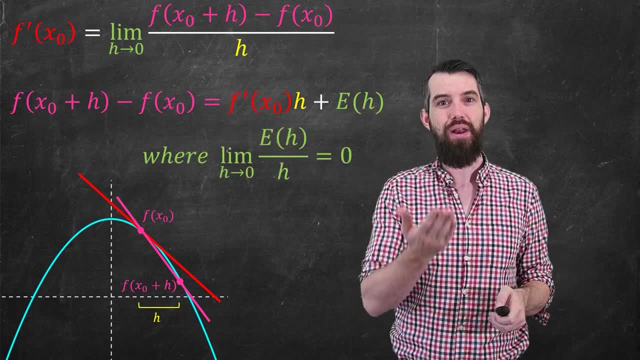 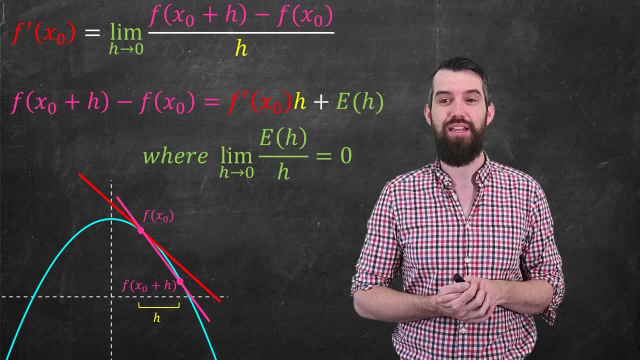 e of h, which stands for an error term, And I'm going to have the condition that that error term, that e of h, is small, In the sense that even when you divide out by that h, even when you divide out by that h, 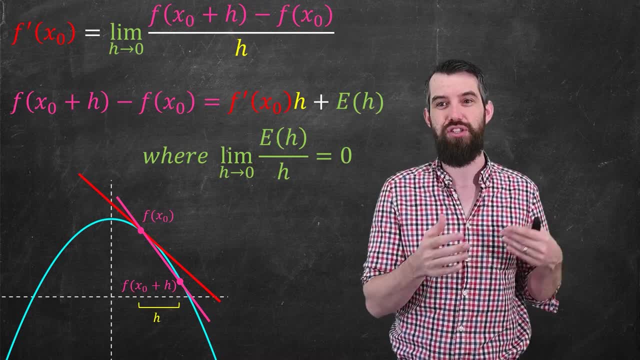 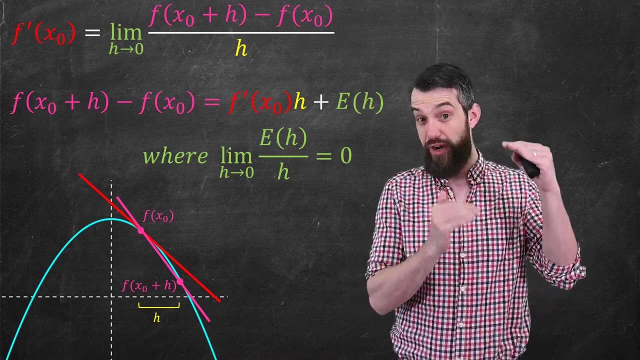 this error term is so small that it's going to zero, as h goes to zero. Okay, so really, what is this error term? Basically, the idea is, when you think about the difference- the f of x naught plus h minus the f of x naught- that is an actual difference on the actual function. 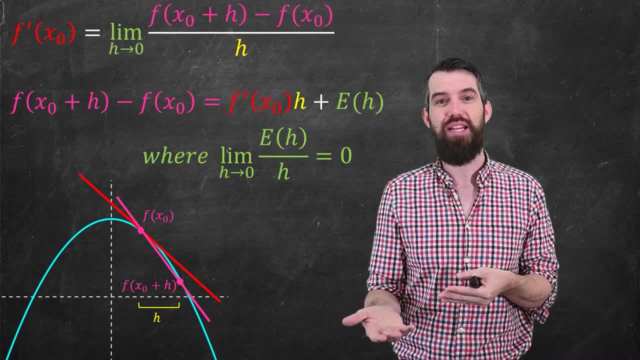 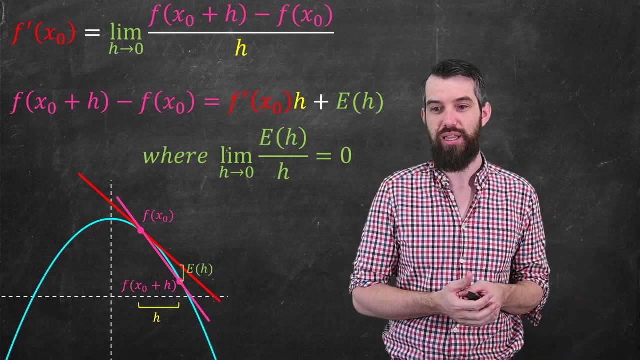 an actual difference heights. You were approximating that difference in heights by the f prime of x naught times h and the error is just the error between those. So on the actual graph what it looks like is the difference between the value on the actual function and going up to that tangent line When 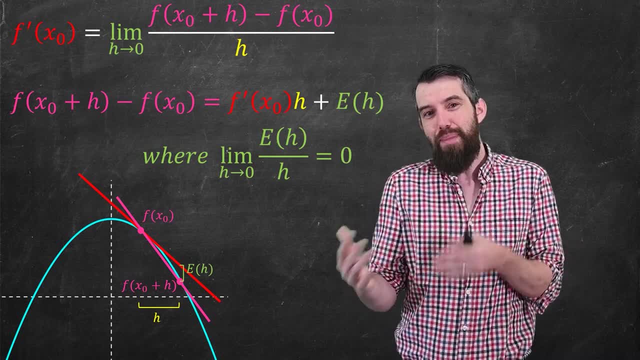 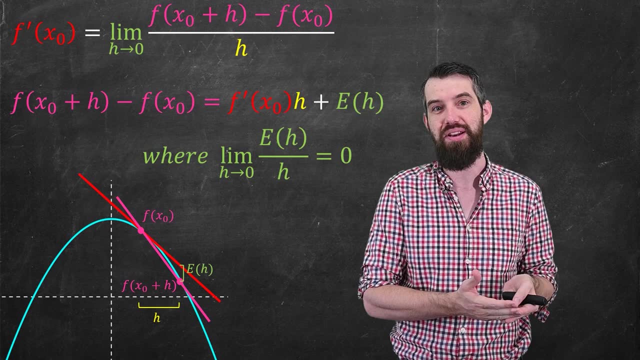 you approximate it by the tangent line. how much of an error are you making? So, mathematically, these two statements are just the same thing. It's just different ways of trying to write down the limiting process. One writes it explicitly at the front and the other has an error term. 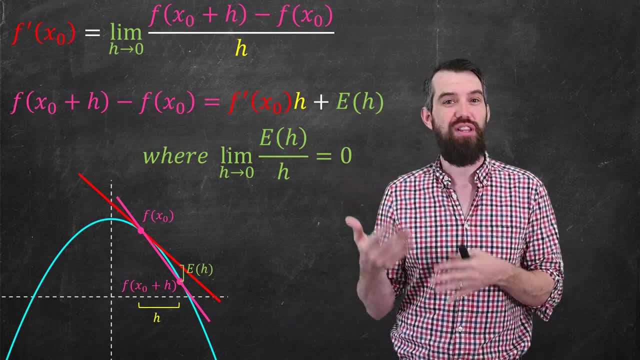 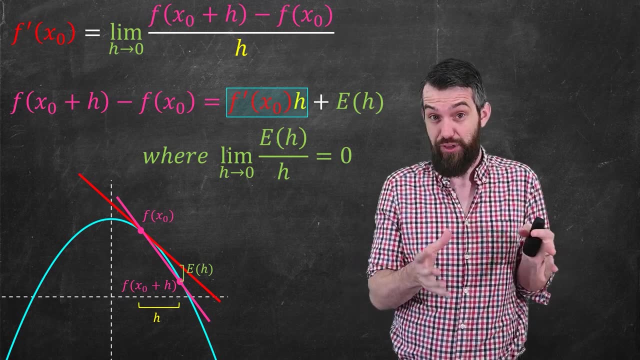 that goes away. Other than that they're the same. They have a nice little philosophical shift in perspective. In this new way of thinking about it, with errors, I can say that I really have this difference approximated by some approximation. That's what the f prime times h is. 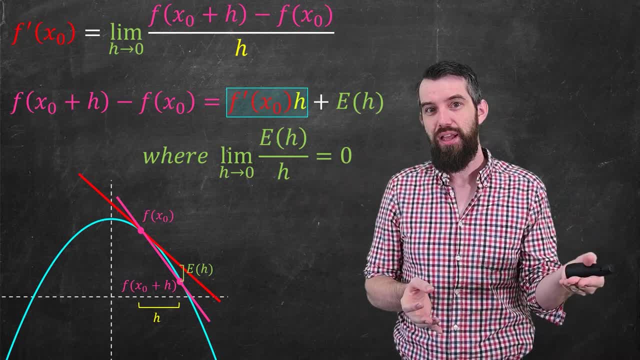 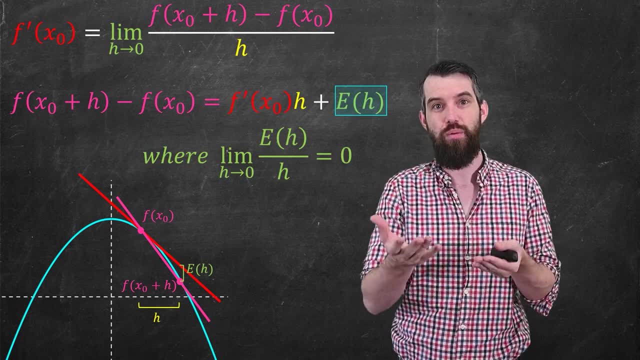 It's an approximation for the amount of change. and then that approximation for the amount of change is not completely accurate. It's got some error term and that error term e of h is what we have here, and the error term is if it's differentiable. 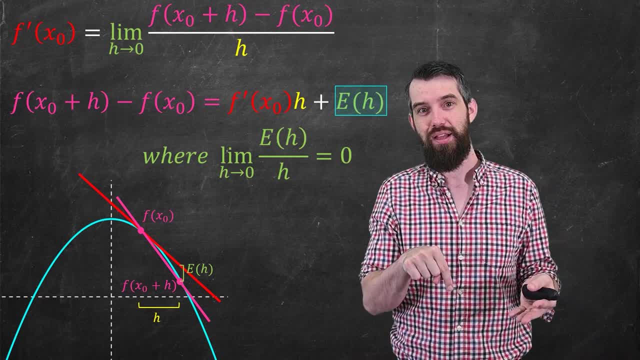 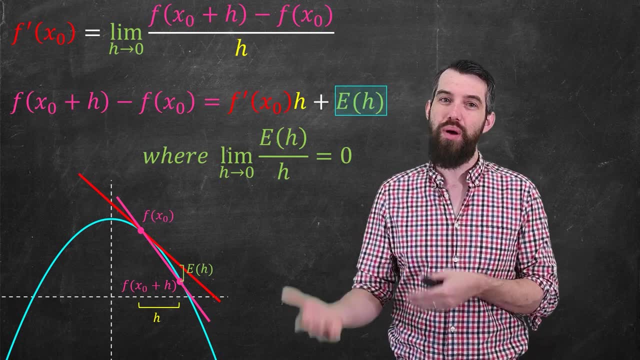 something so small that even when you divide it by h, which is going to zero, that the limit is still going to be equal to zero. So a very small error term, at least when h is very small. Okay now, the reason why I'm going back to the single variable calculus case is we wanted to 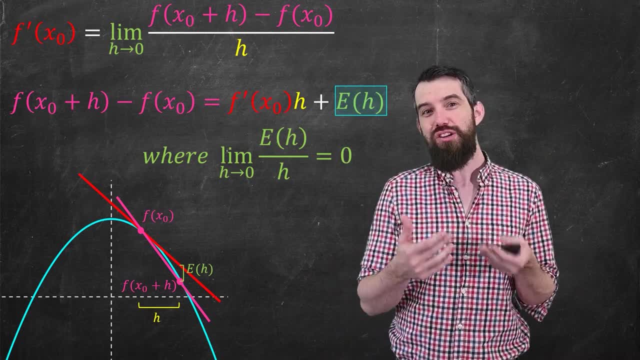 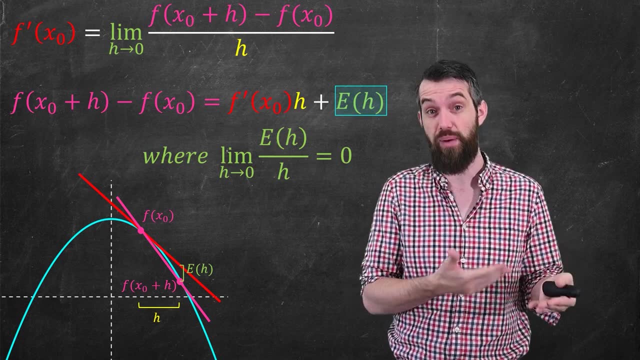 get to multivariable differentiation, and I'm actually going to use the second of these two perspectives to come up with my definition of the differentiation of a multivariable function. So let's jump now to a multivariable function. It's almost exactly the same. 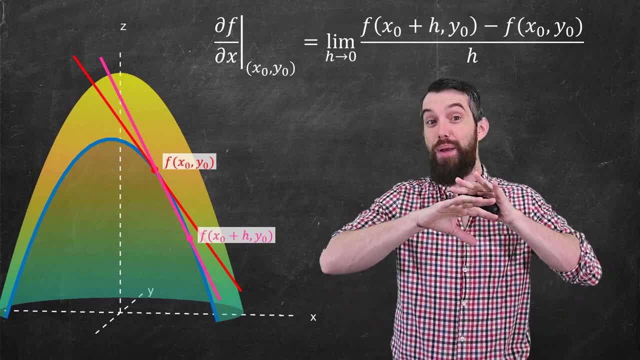 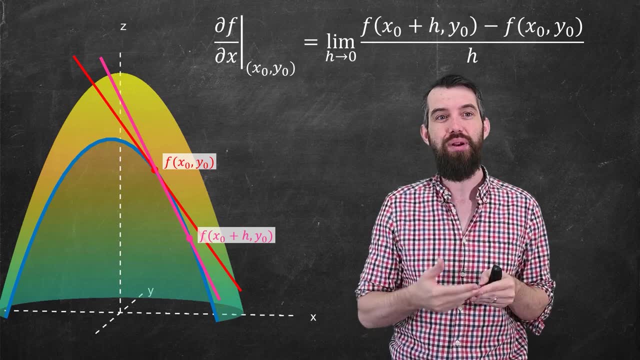 except instead of 1 minus x squared I have the 1 minus x squared minus y squared, so I get this nice surface. And then what I'm doing here is I'm considering some point, not just x naught, but x naught comma, y naught, at point in two dimensions, And the formula I've put 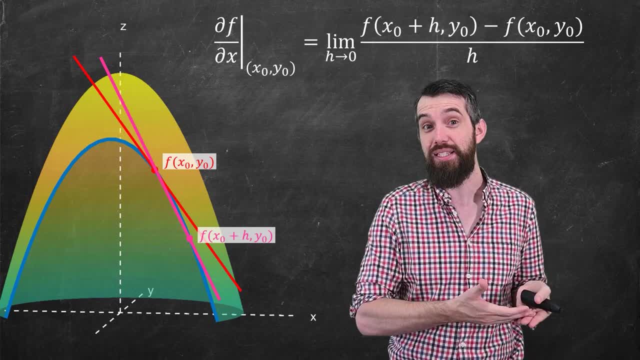 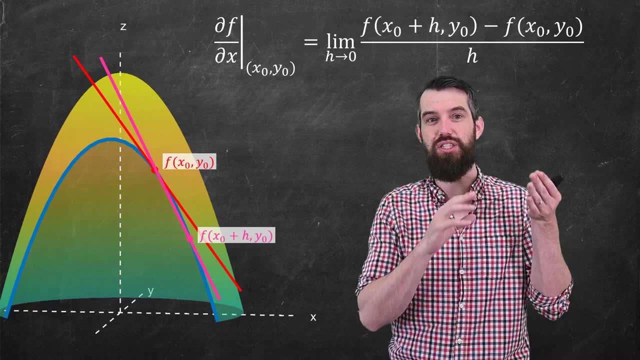 up here is the partial derivative of f with respect to x, at the point x naught, y naught, And indeed, again, it's defined in the same sort of way that we've seen in the past. it's just the limit as h goes to zero. 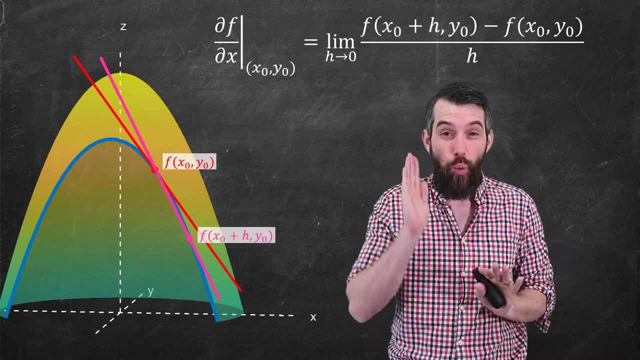 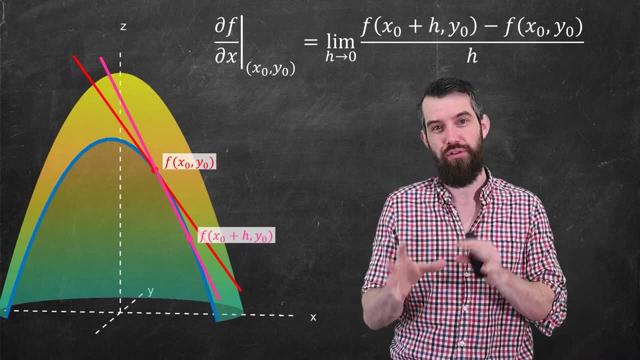 in the y component you say it's a partial derivative of x. we're keeping y fixed, y doesn't change, just y naught. But in the x component it goes from x naught to x naught plus h in your difference quotient And then visually we get basically the same picture we just had. 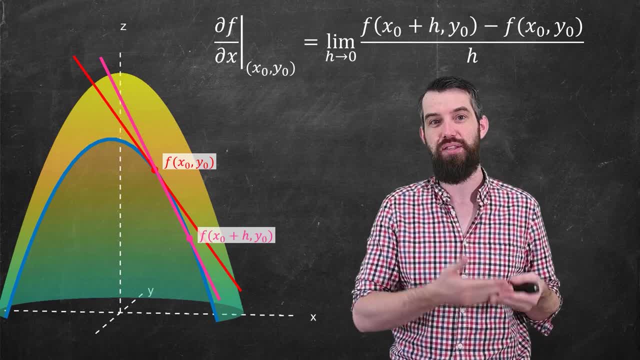 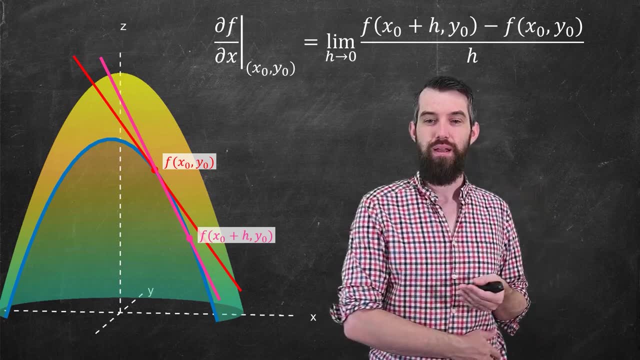 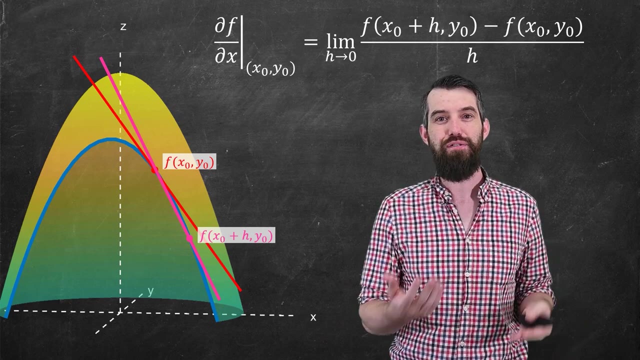 the pink lines represent the secant lines, and the slopes of the secant lines approach the slope of the red line, which is the tangent, as h is going to zero. So partial derivatives and derivatives of single variable functions are really very similar, and the reason for this is that a, 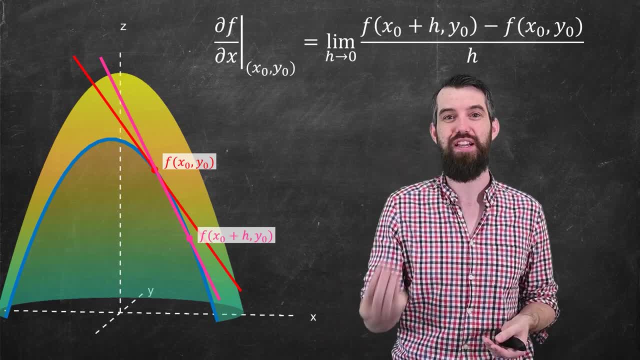 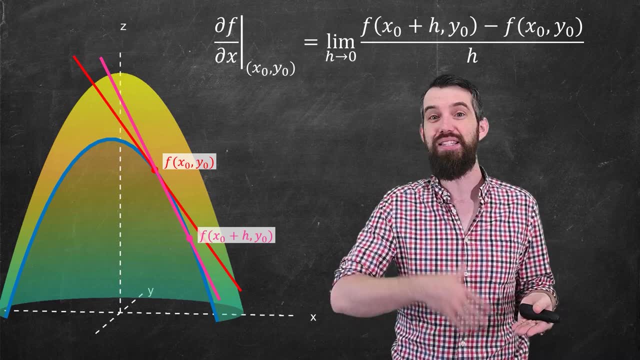 partial derivative just says: let's just fix the y value. imagine it's just a fixed number and then the function just becomes a single variable function. it's only x that's changing, and so the pictures really align very nicely. I did this for the partial derivative with respect. 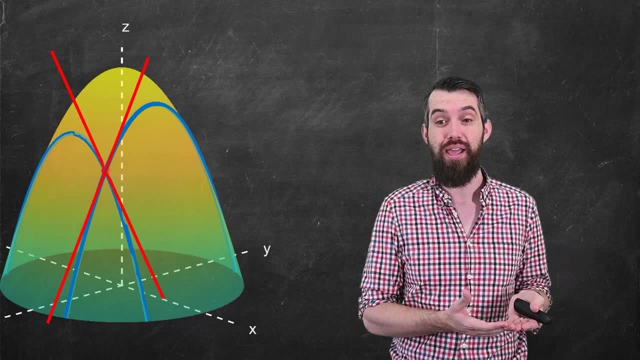 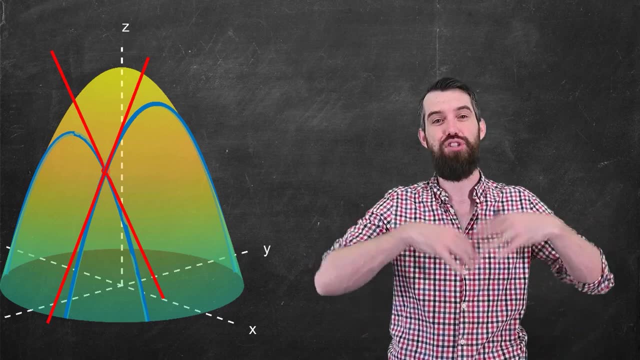 to x. but I mean, we have a partial derivative with respect to x and y At your point. x naught, y naught, you can slice with respect to x and you can slice with respect to y. you get sort of two different curves. they each have two different tangents. those are the partial derivatives with respect to x and y. 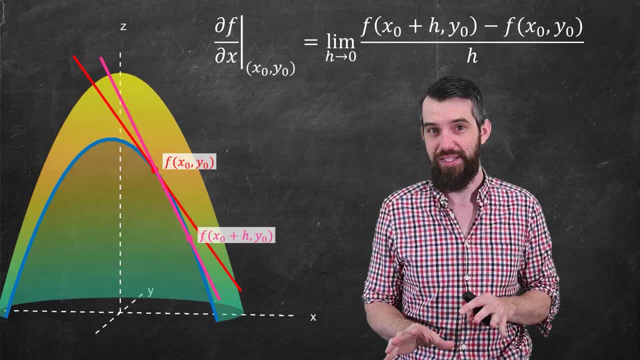 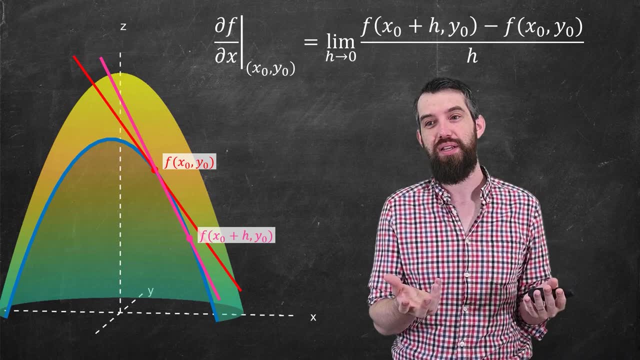 and then the partial derivative with respect to x. Now let's go back to just focusing on the one with x. I now want to do just a very slight shift of notation. I'm going to be imagining changing x and y in a moment. so instead of having h as the symbol for my little change, I'm going to take 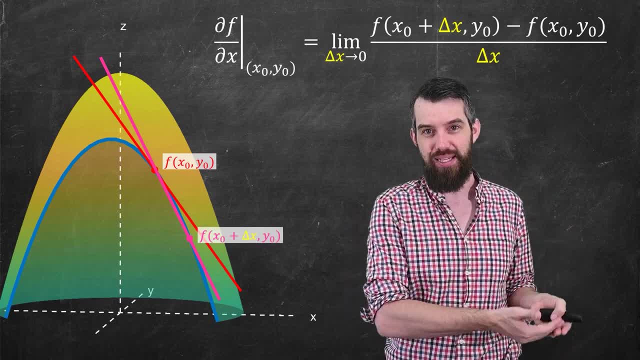 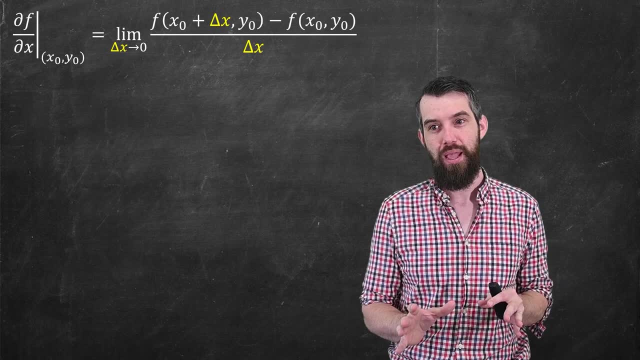 all the h's and I'm going to replace them with delta x's instead. The argument here is that I'm going to have a delta y in a moment. Okay, so let's get up some space here. so I've got my expression, and now what I want to do is I want to rewrite this. 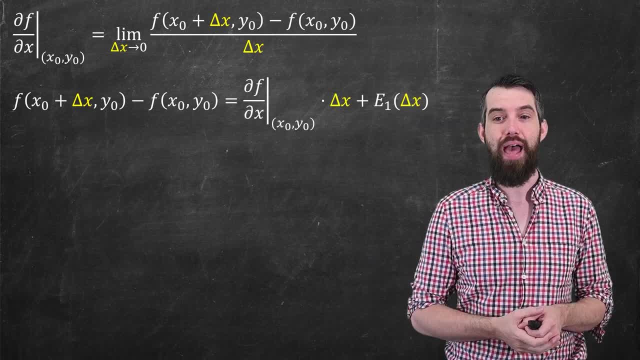 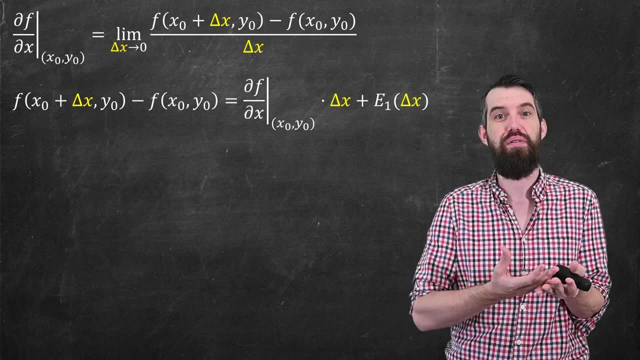 in terms of errors, just as I did previously. So okay, doing that looks like the following: The difference is now the thing you approximate, that's that partial derivative times a delta x plus an error term. we'll call it e1, because we're going to have two error terms in a moment. 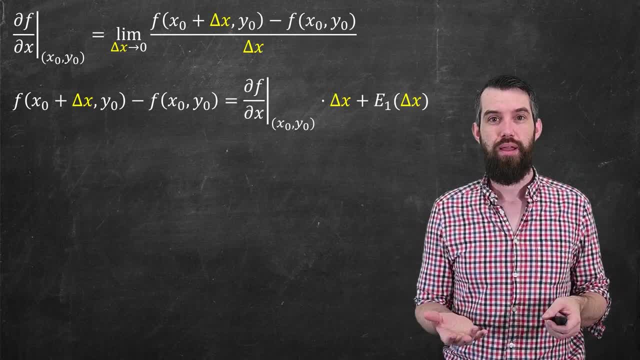 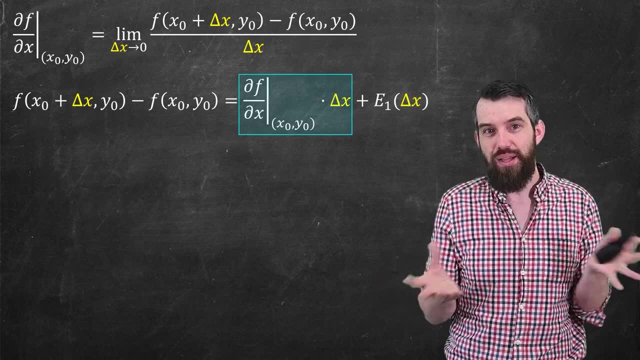 the error term. that is a function of delta x And indeed I really do want to think of this rewriting of that formula as having this approximation term. that's what the partial derivative represents and it's a function of delta x. So I'm going to take that and I'm going to 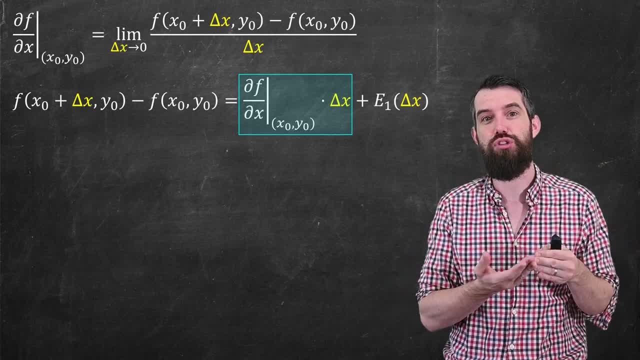 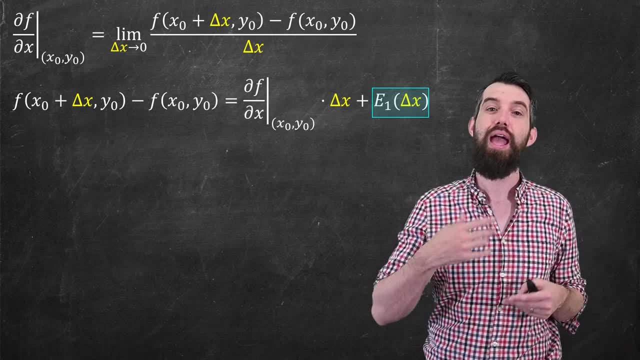 put in here delta x, It's approximating the change that you're going to make when you shift over by delta x, And then that approximation term is still an approximation because it's also got this error term And we've seen that the error term needs to be small in an appropriate sense. Okay, so that's. 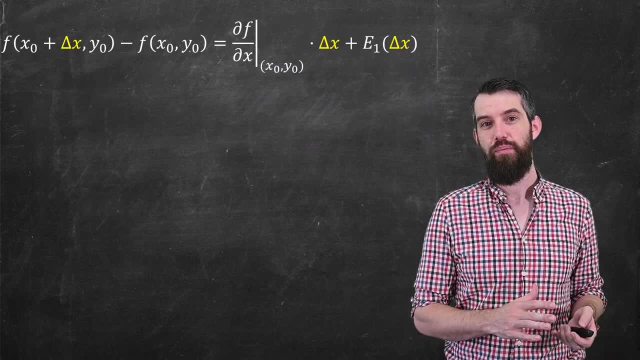 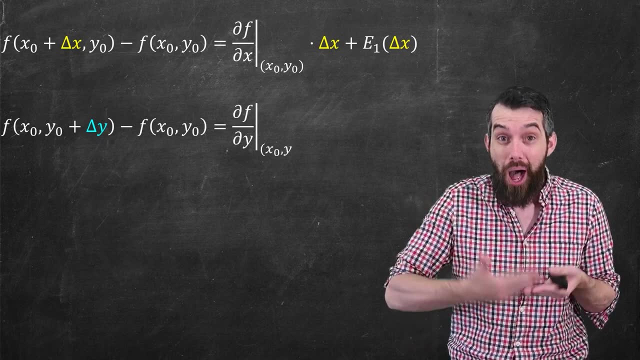 the partial derivative with respect to x. Let me put it just there by itself, But we could also write down the partial derivative with respect to y. It's going to be the exact same story. it's just that the y naught is changing to y naught plus delta y And as a result, that you're. 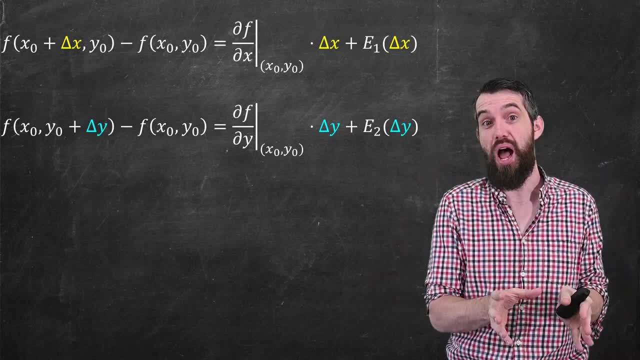 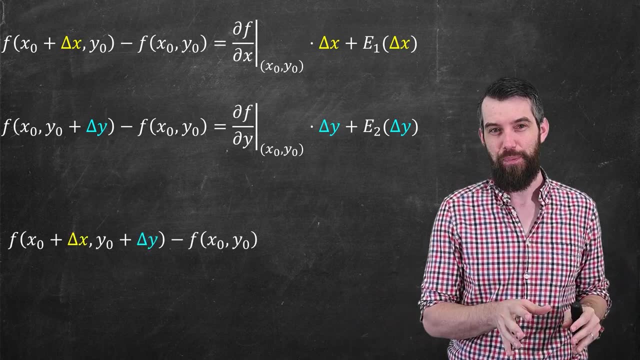 you're going to get this approximation in terms of the partial derivative with respect to y and then an error term in terms of delta y. Now here's the big moment. Here's the moment we actually get to differentiability. So I want to consider a difference where I am now changing. 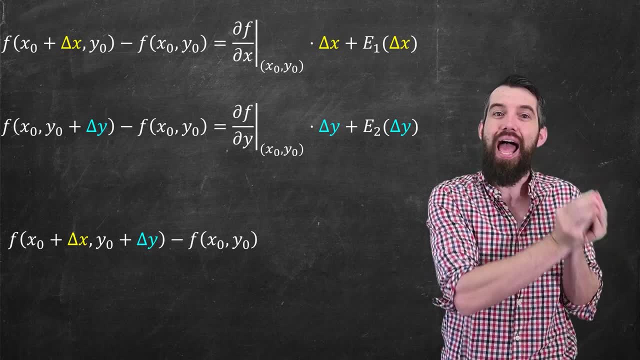 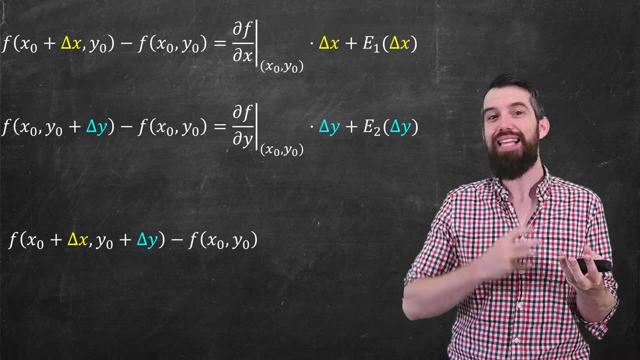 the x-naught, y-naught to x-naught plus delta x and y-naught plus delta y, As in what's changing here is- I'm imagining both the delta x and the delta y. change that. I'm taking my one point and 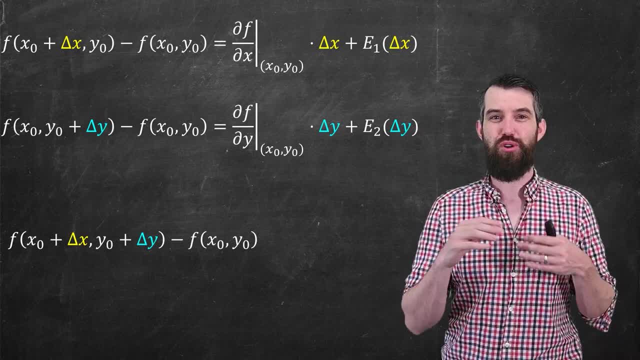 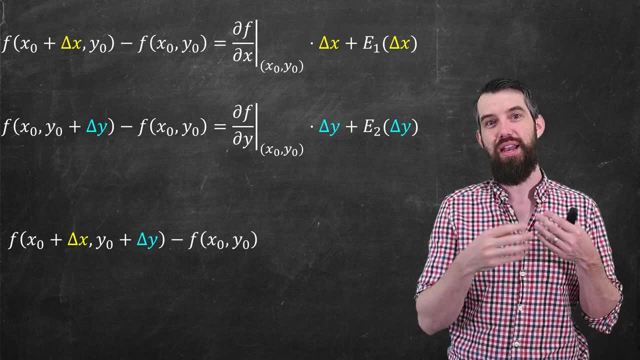 moving it in two different directions at the same time. The sort of problem with partial derivatives was they sort of were too restrictive. They only look when you're changing x by itself or y by itself, and now we really want to think of both of these things changing at the same time. So the 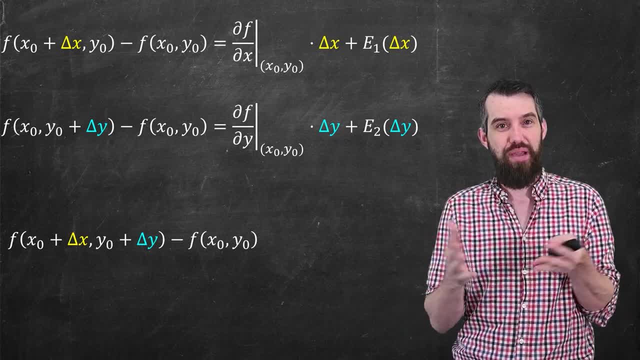 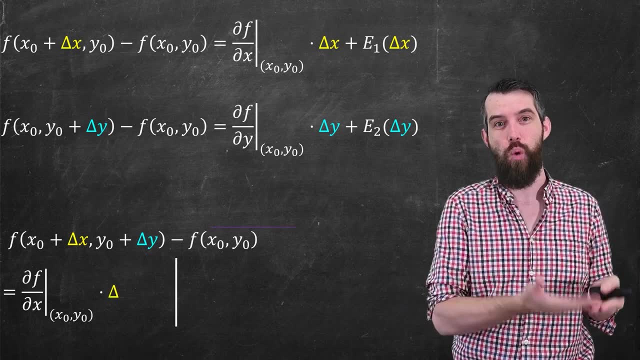 argument here is that when you change x, well we have this approximation in terms of the partial derivative with respect to x that you get. When you change y, well we have the approximation of the effect that that has in terms of changing y. So what if I set this to be the sum of those two? 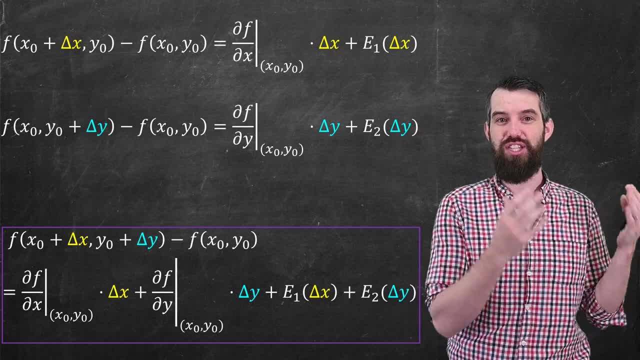 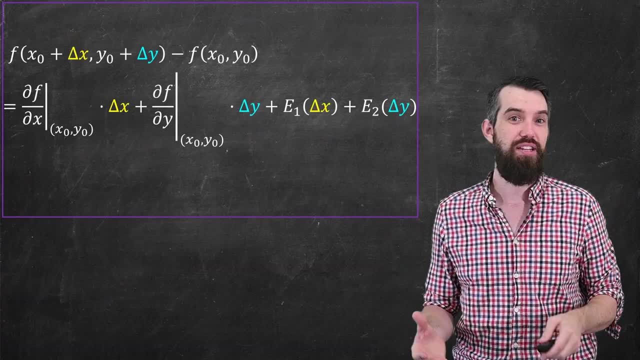 things. So what if I set this to be the sum of those two things? That is, I have a component which is the change in x and the component which is the change in y, and the error from changing x and the error from changing y. Indeed, if I had just a couple more. 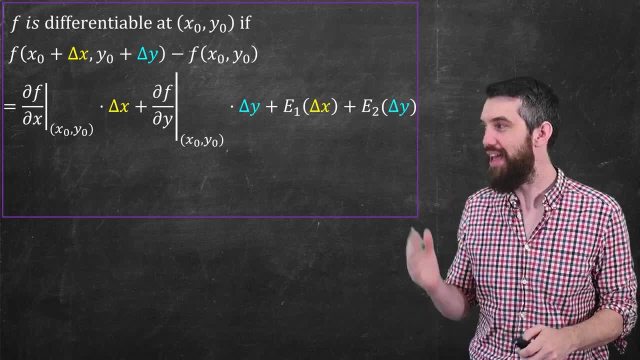 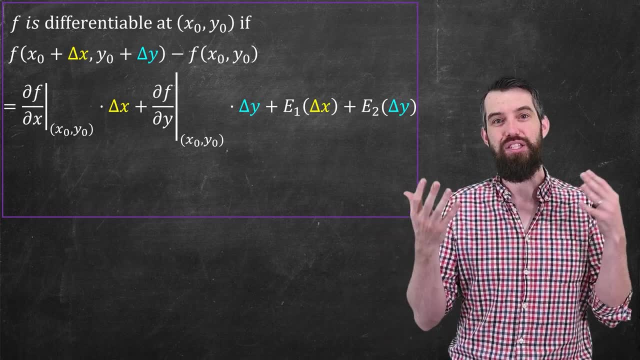 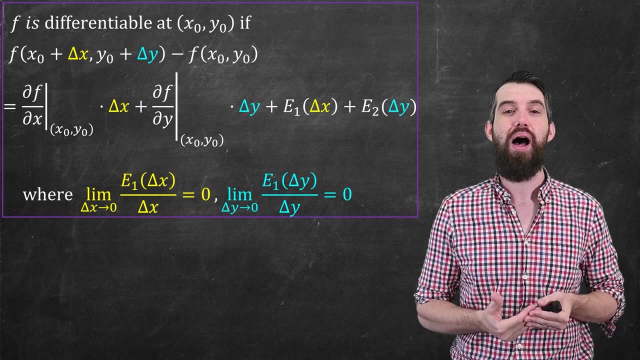 things. let me just give myself a bit more space. I will now formally define that f is differentiable at some point, if this long expression that I have is true, and that the errors are appropriately small. In other words, I need to say that the limit of the e1 divided by the delta x is zero. 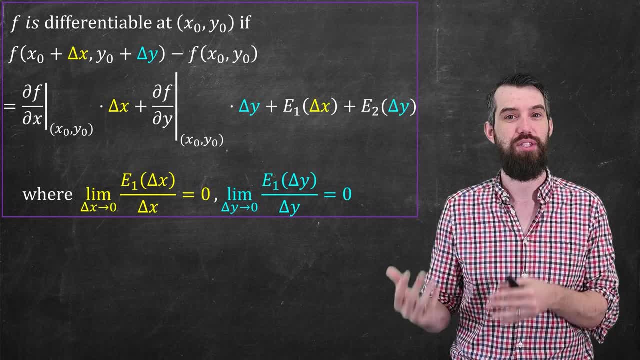 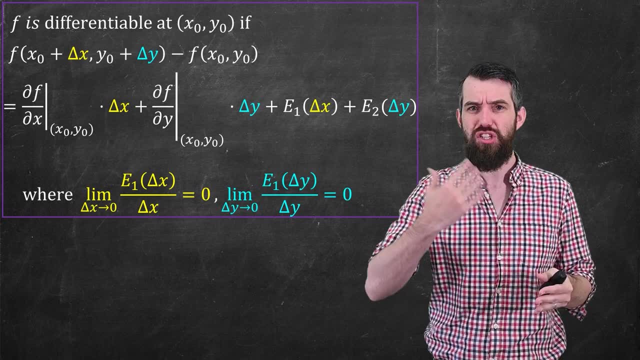 and that the limit of the e2 divided by the delta y is equal to zero. I need to have both of those things being true. So that is my definition of differentiability, And actually let's just walk through it one more time just to make sure we're all confident. The first thing we want to focus. 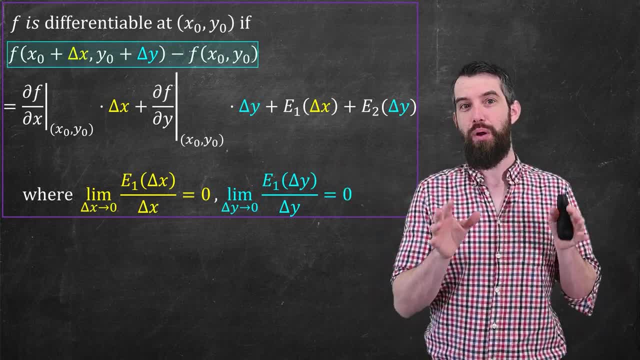 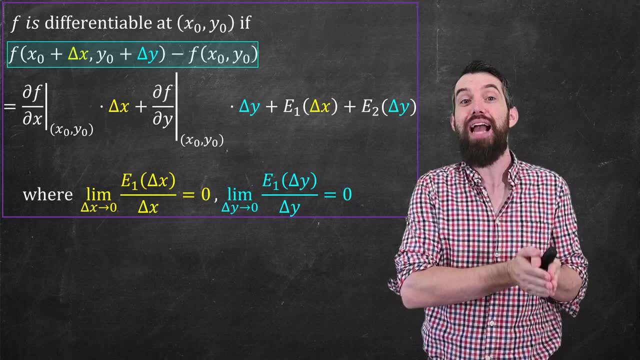 on. is this difference? That's what I've been studying all along. I want to know what is the difference between the function when you change from one point to another, In this case x naught y naught to x naught plus delta x and y naught plus delta y, And then what we're seeing is that 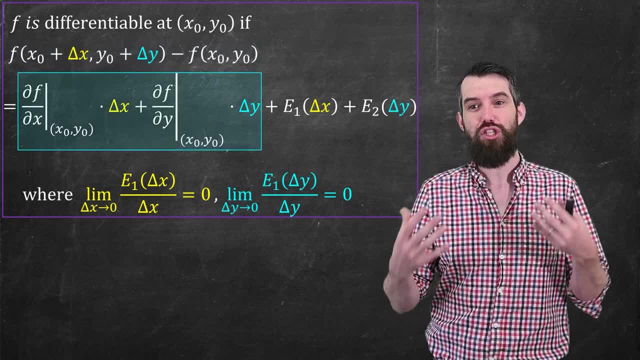 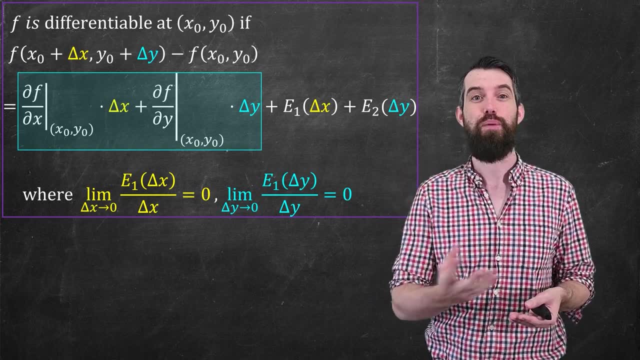 this difference can be approximated by these two expressions with partials. There's the change with respect to x, The partial derivative with respect to x times the delta x. That's sort of the approximation of the contributions from changing x. And then we approximate the 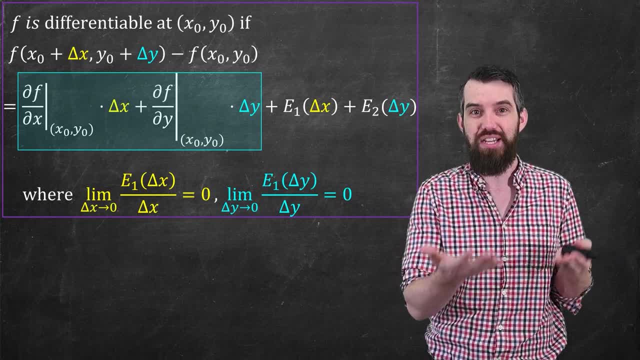 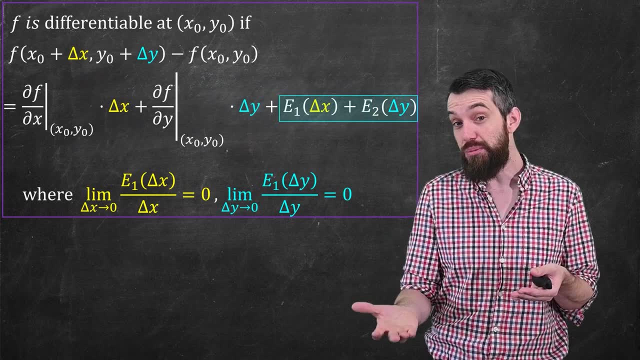 contributions from changing y by the partial derivative with respect to y times delta y. These are approximations, so they have two error terms. There's an error term from the approximation in terms of x and in terms of y, But these error terms are small in the. 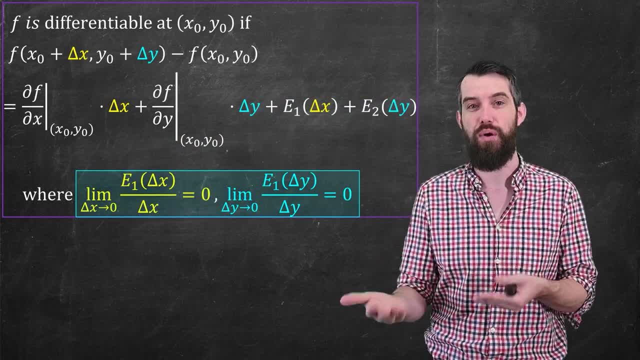 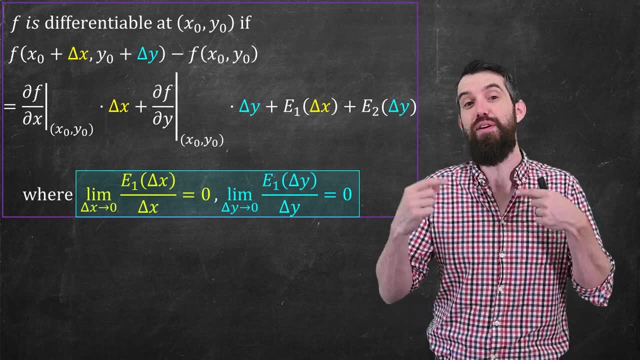 sense that these of these error terms are both going to 0. In fact they go to 0 fast, Even when you divide out by delta x or delta y, which are themselves going to 0, even then they're still going to 0. So these error terms have to be really small, at least. 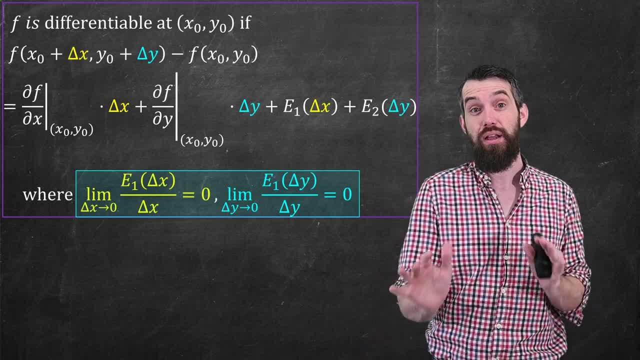 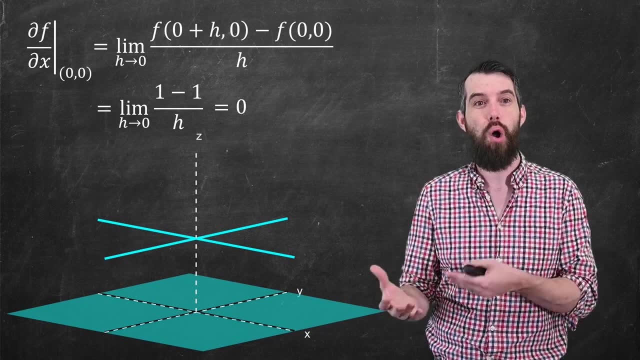 as delta x and delta y are going to 0. If you have that, then you have differentiability. Alright, let's see an example. I actually want to return to this example that we saw in the previous video of the cross and I'll remind you. 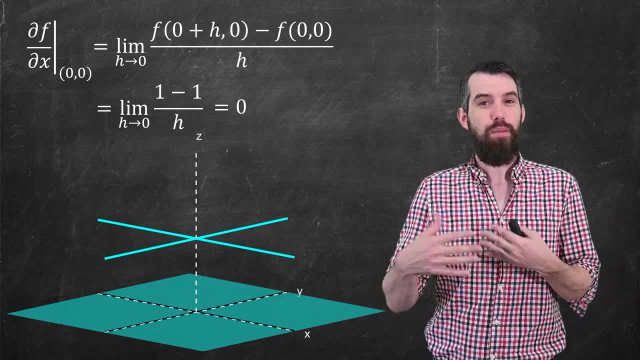 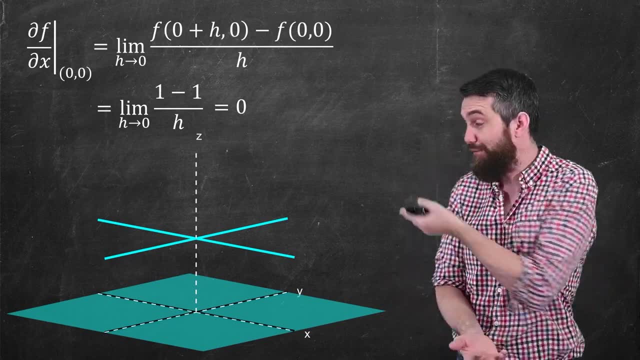 that this example is a discontinuous function but that the partial derivatives both exist, Because when you look down the one axis or look down the other axis, the function just looks like one. there. It's defined to be one along the axes, And so according to the partial derivatives, and that's the computation I. 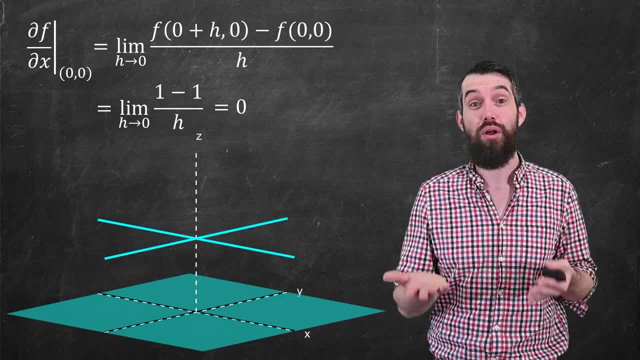 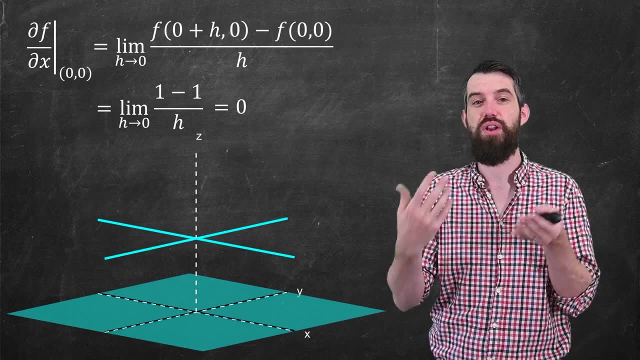 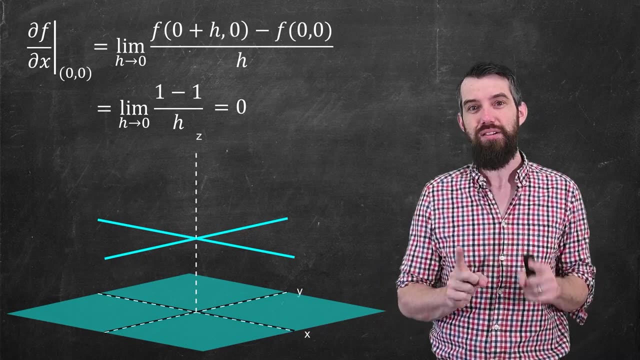 put up here the partial derivatives, think this is just a horizontal slope of 0. And that was a problem for us because it sort of violated our intuition that discontinuous function should not be differentiable. But here this discontinuous function had existing partial derivatives. But here's the issue. If I focus in on what's happening, 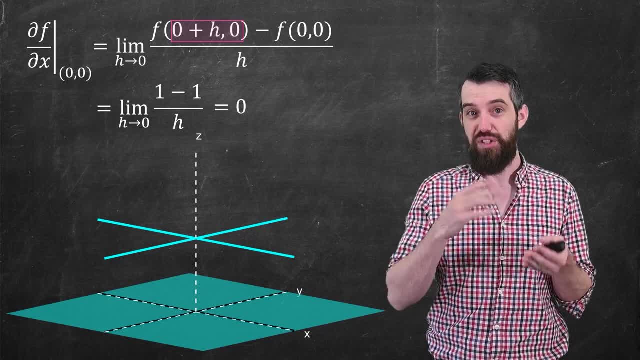 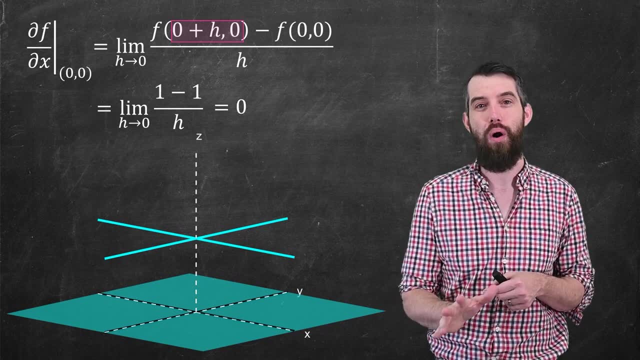 on the shift, when I only change in terms of h, this f of 0 plus h and 0, well, what's happening there is? it's quite a special case because I did not change the y at all. If I imagine a change in x and y, like we did in the definition of, 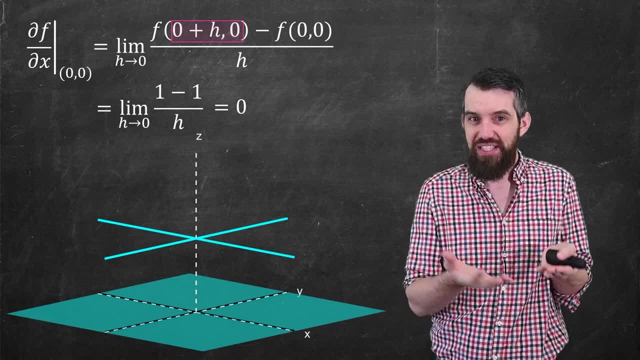 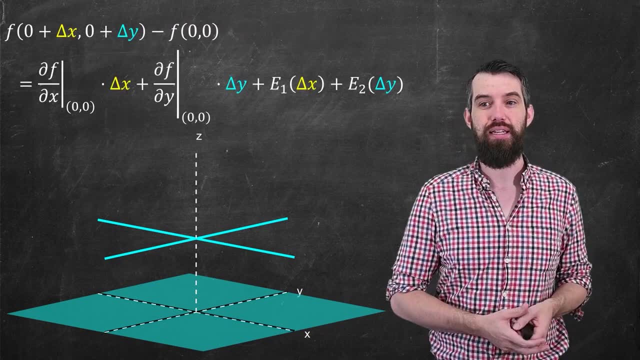 differentiability, then it would shift off the axes now because both components were changing. So those are the special case of partial derivatives, And the shift of partial derivatives is about to go away. Okay, indeed, let's go and try to do this by writing out that definition of 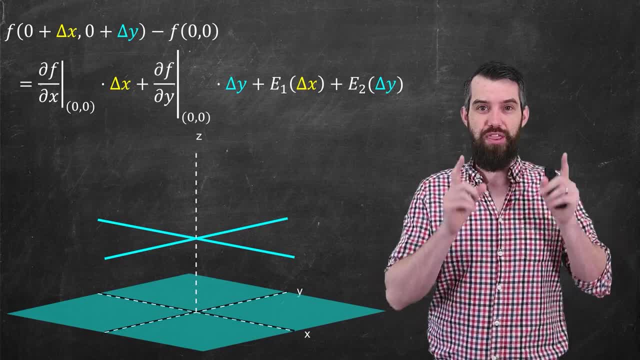 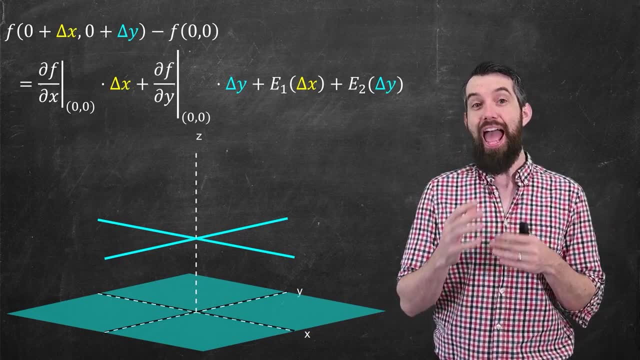 differentiability and we'll see whether or not the error terms are indeed small. So I put this all in The point- is 0, 0.. The shift is delta x and delta y And I've got this expression for the partial derivatives As we computed both partial. 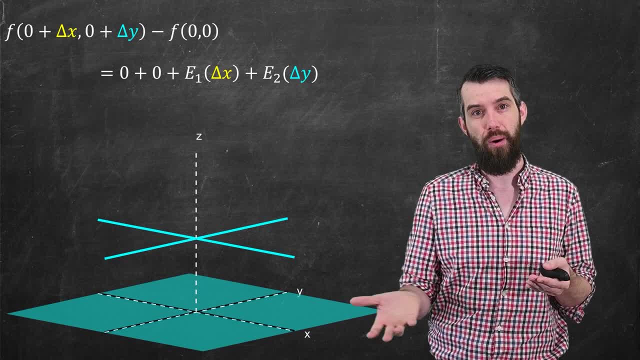 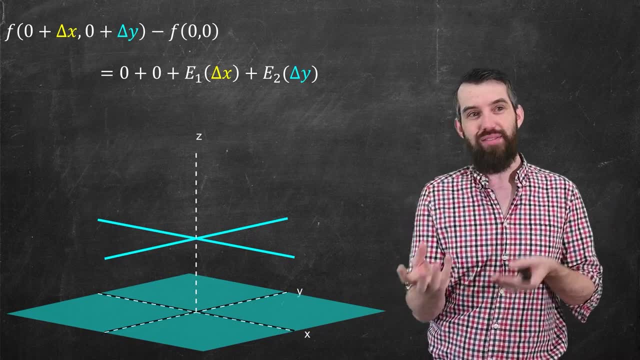 derivatives are 0. So I can simplify this a lot by getting rid of those partial derivatives and it's just a 0 plus a 0.. The difference, well, f of 0, 0 is 1. And f of delta x, delta y. this is generically. 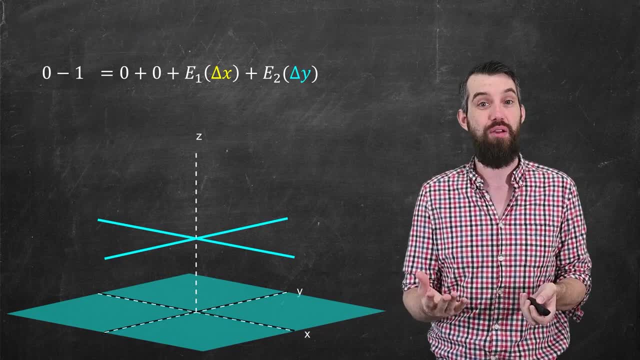 some point which is not on the axes. So generally it's going to be well 0 because it's not on the axes. So what I have on the left is 0 minus 1, minus 1.. On the right: 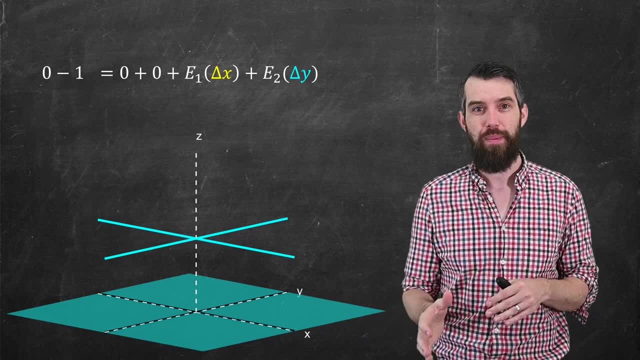 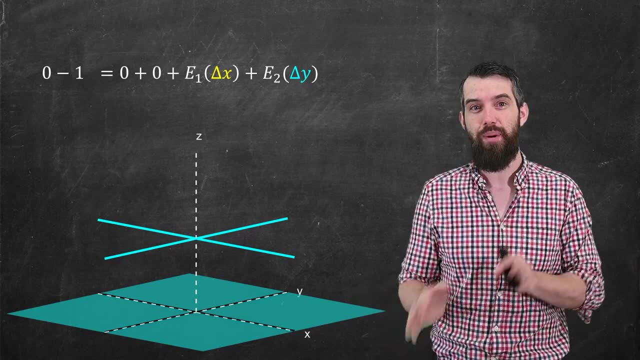 I just have some two error terms. Now here's the point. Those error terms, if it's differentiable, have to be small And the limit, as delta x and delta y are going to 0. But they cannot be small because they have to add up 2 minus 1.. 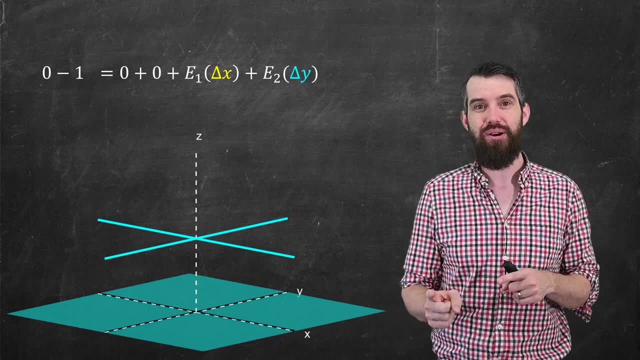 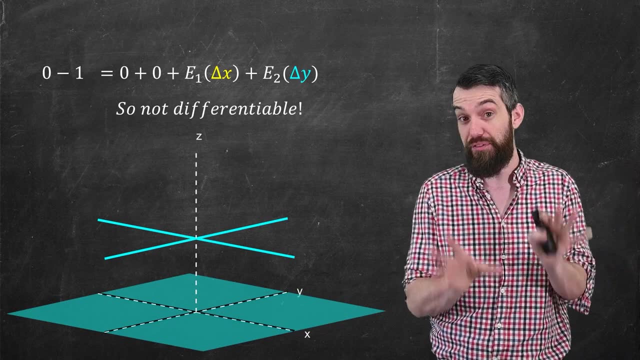 Minus 1 is not close to 0. So the point here is that these error terms cannot both be small And as a result of this it's not differentiable. The attempt to write down that formula for differentiability did not give small errors, And so it was not differentiable. 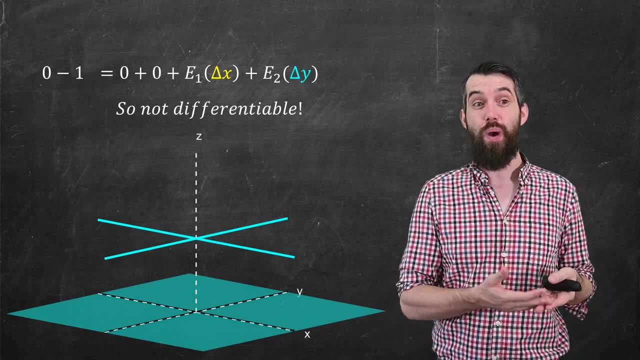 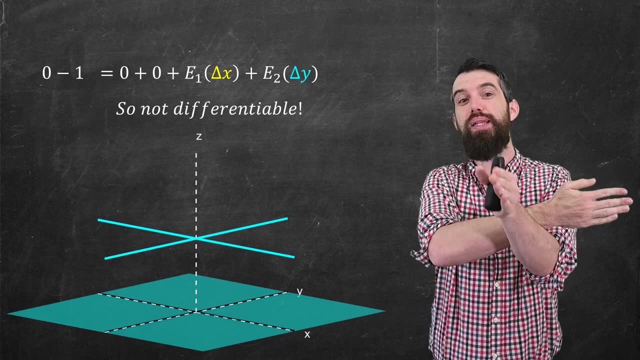 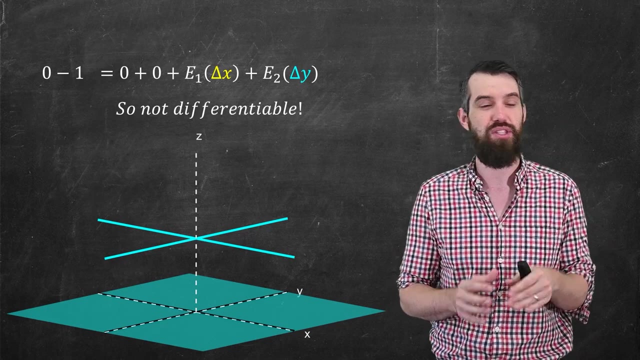 So now we resolve the tension in our story. Well, the example previously had a discontinuous function with existing partials. We now see that it's because partials are too limiting, They don't see the problems. Differentiability- the full differentiability does see the problem here And so this discontinuous 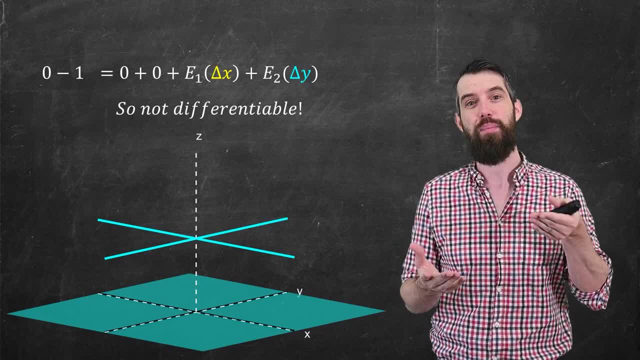 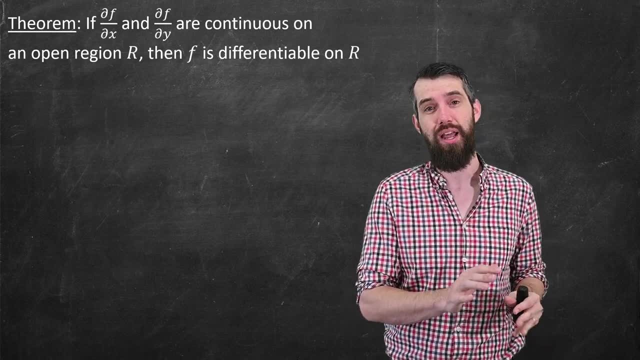 function is not differentiable as we would have expected from calculus 1.. So I might have left you with the sense that partial derivatives are a bit useless, But in fact they still are. And they still are because of this very powerful theorem: It.